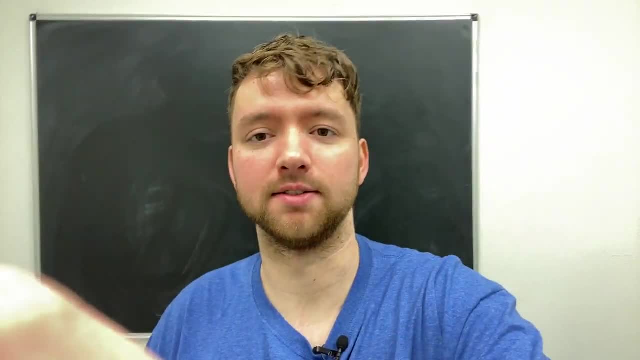 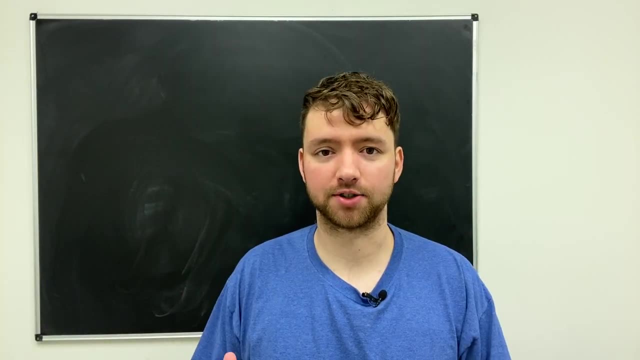 I'm just playing. I just haven't fixed the settings yet. Let's try to get these looking a little bit more normal. There we go. So what are we going to be talking about today? We're going to be talking about the stack data structure. And yeah, I just like looked because 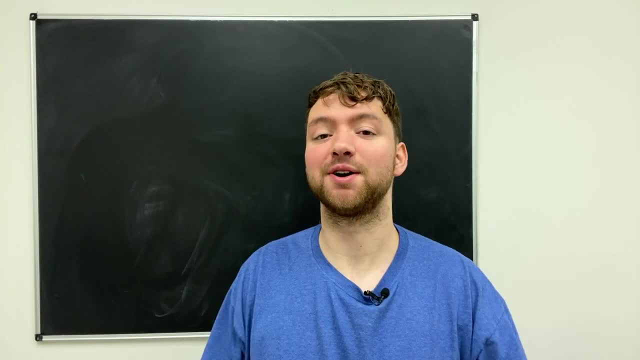 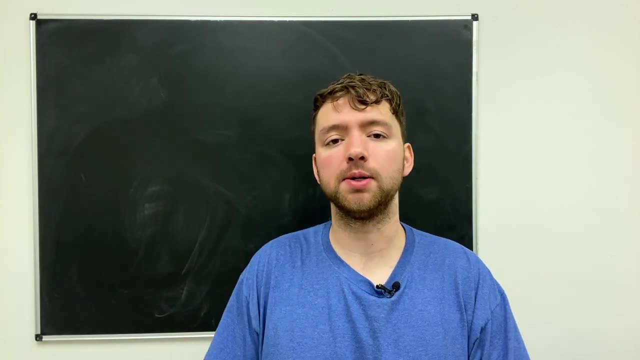 I couldn't remember, So I have my notes over there. So we're going to be talking about stacks, So these are often taught with another data structure known as queues. They're very similar, but it helps to understand stacks first And then picking up the queue is actually a piece. 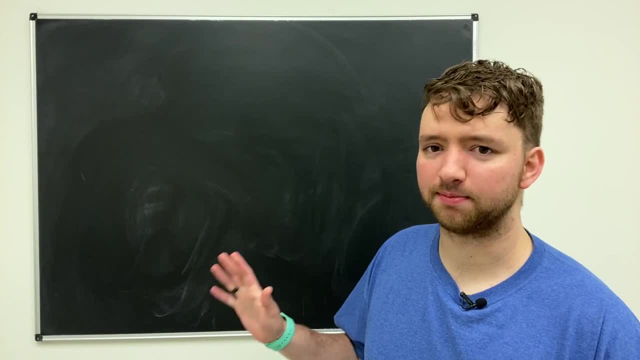 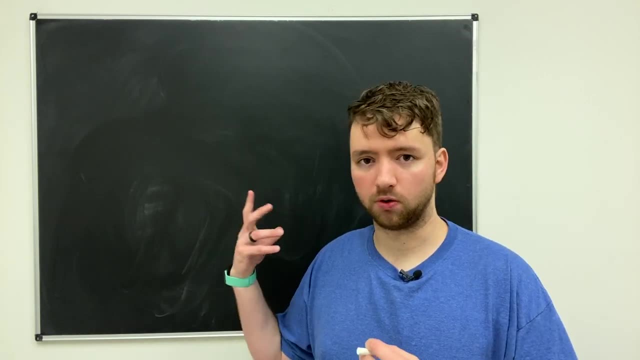 of cake, And no, I don't mean a literal piece of cake, I just mean it's going to be easier to learn the queue after you learn the stack. So let's get started. So the way a stack works is first. we're going to approach it more like a conceptual way And 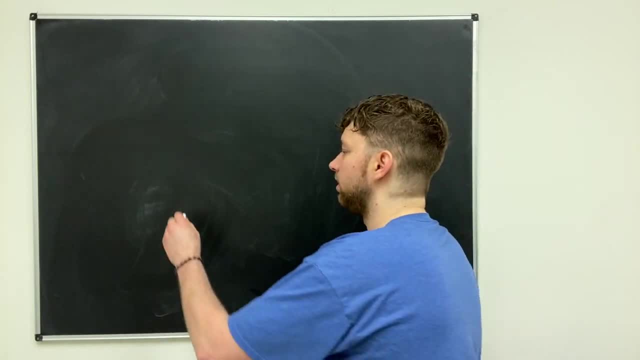 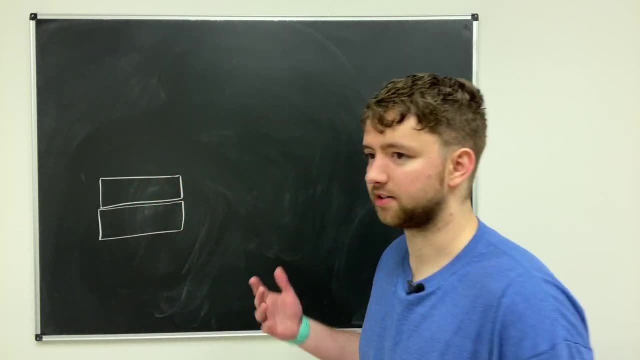 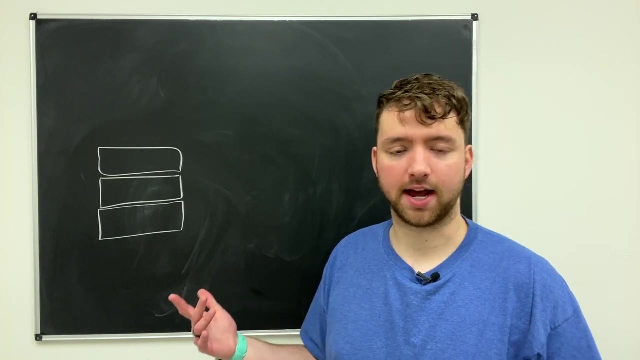 then we're going to look at some of the operations of a stack. So in the example of, let's say, books, if you have a stack of books- and I literally just mean a stack of books, nothing technical or fancy here- Well, if you wanted to add a book to this stack, the most logical place to put it. 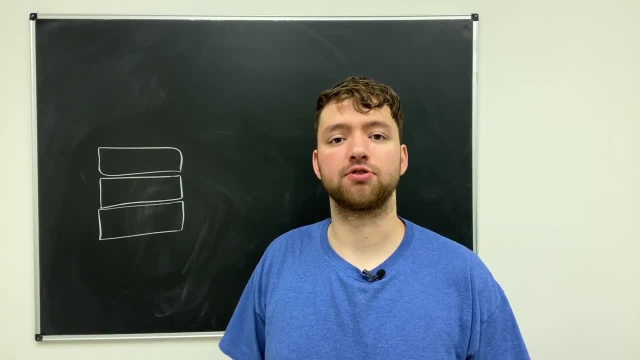 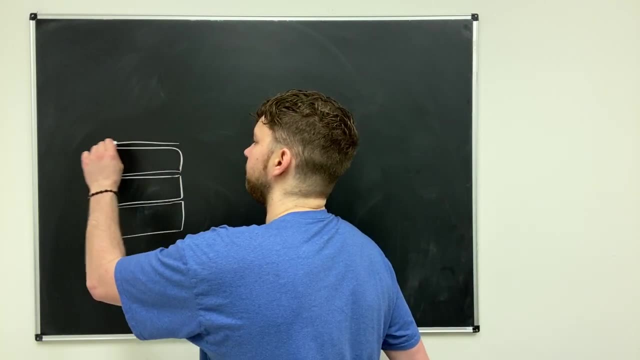 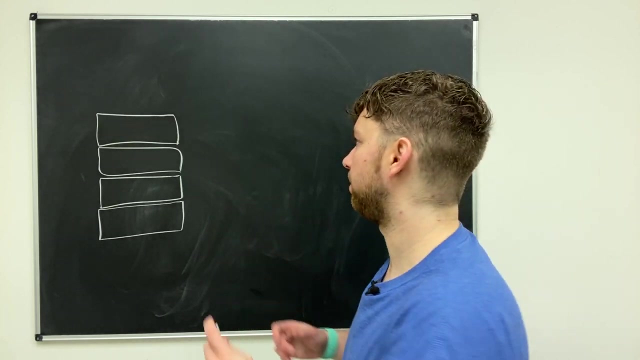 is on the top, And that is how a stack data structure works As well. we're going to represent data in such a way that we put stuff on top, like so, And then, when we need to get data back out, we actually take it off of the top. So this one's going to 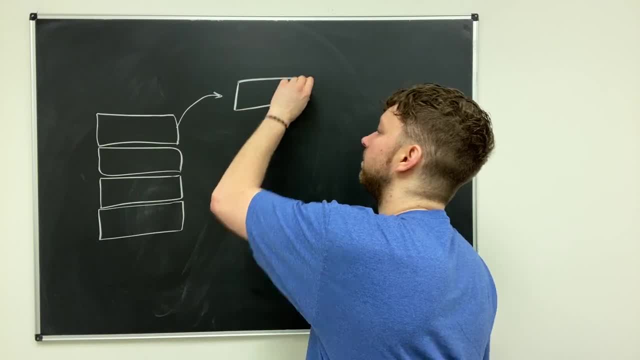 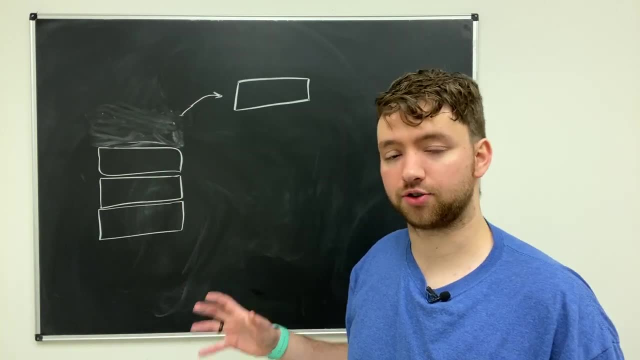 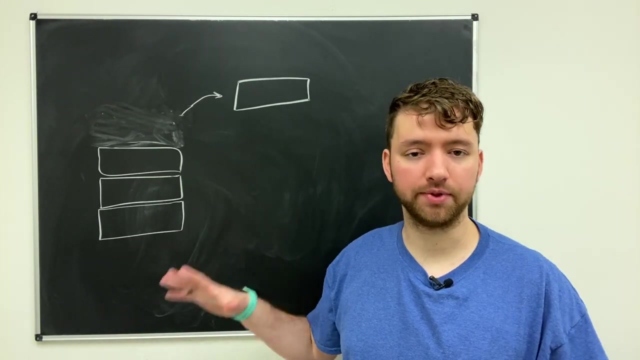 come off of the top and we will have it over here, And then it will no longer be on our stack. So, conceptually, that is how a stack data structure works, just like a normal stack of anything in real life. Now, if we wanted to describe the capabilities of a stack data structure, we could break it down to: 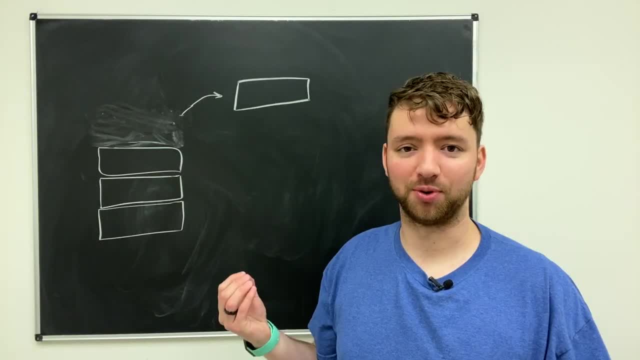 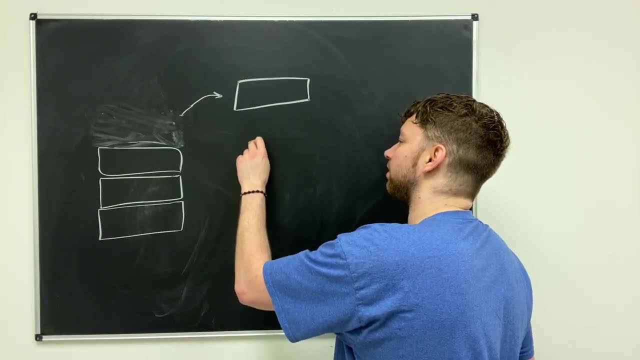 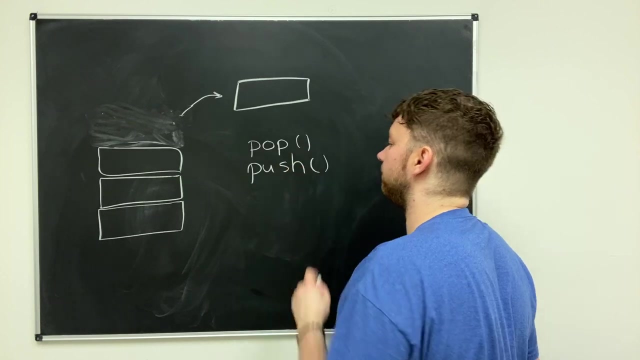 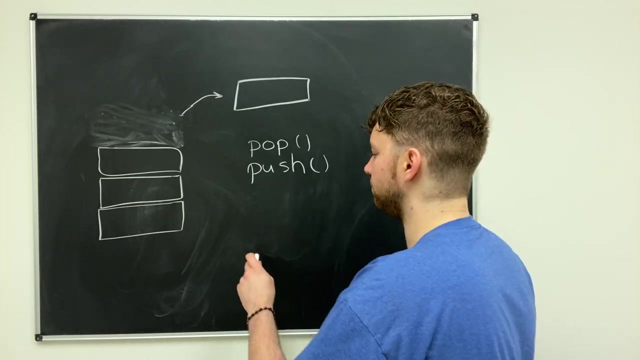 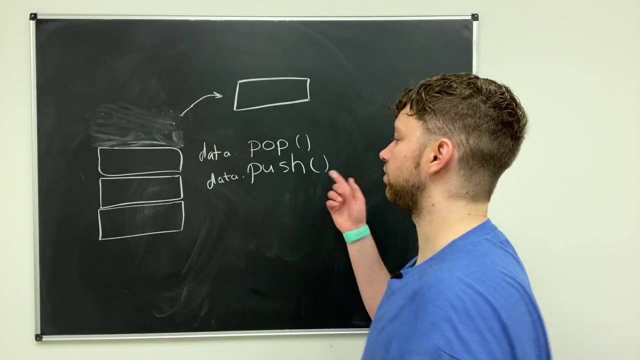 two key, essential, very important operations Had to have as many adjectives as possible there. So these operations are pop and push And these are functions, or actually usually these are going to be methods on an object in our code. So you might have something like datapop and datapush, where data is some collection. 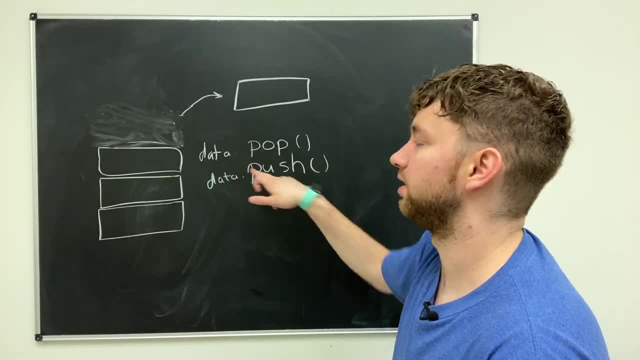 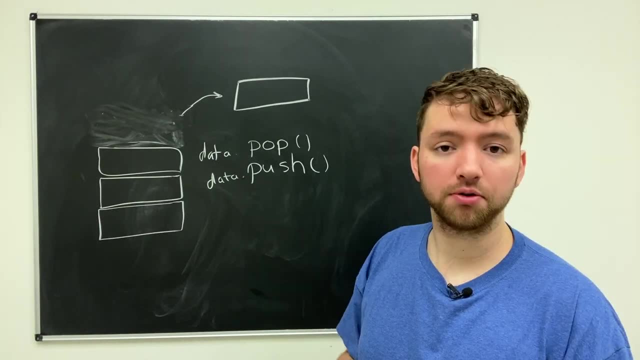 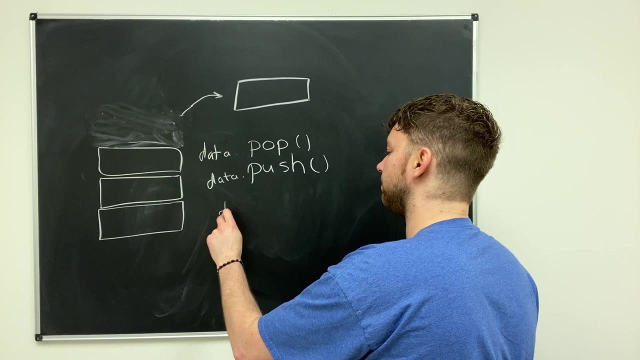 some variable. Now, what is the data type of this data variable? Well, it's going to be some collection, And by collection I mean it's probably going to be a dynamic array or a linked list. So those are the two common ways of doing it. You can do it with a dynamic array. 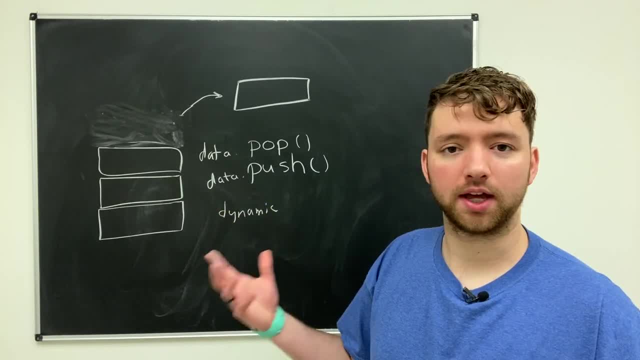 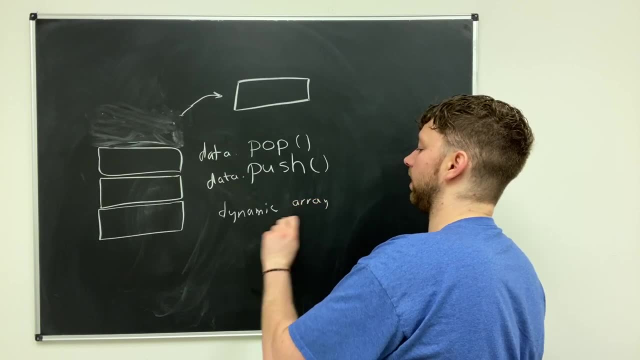 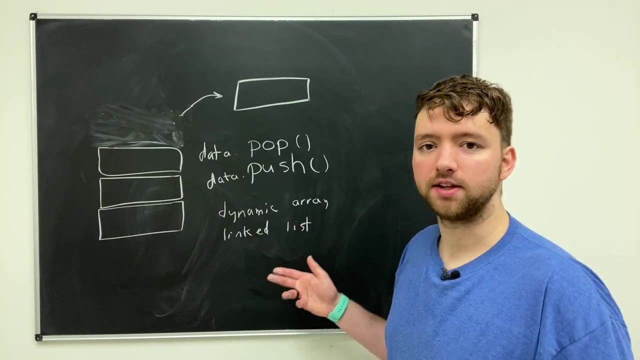 too Heck. you could even do it with a static array too. It's just going to be a little bit different, But most of the time it's going to be a dynamic array or a linked list And heck. this is interesting because there's actually different ways of creating a stack And because 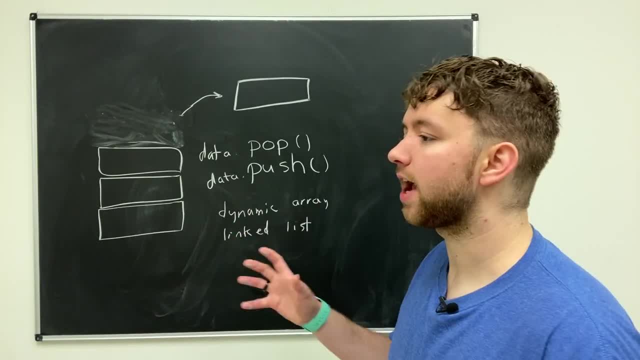 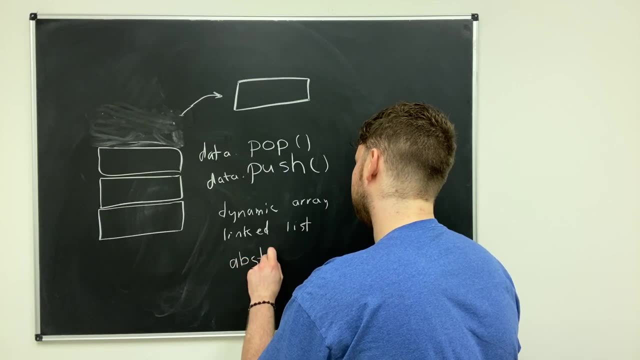 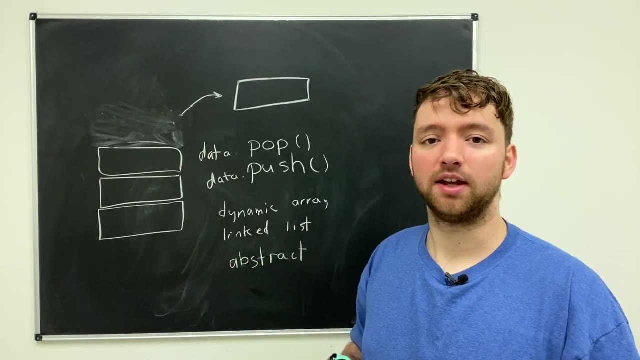 of that because there's different ways of doing it. the stack is known as an abstract data type. So you know, when you study like abstract art, it's just people like splash paint up on something And they say something like: hey, you can interpret it however you will, You can bring. 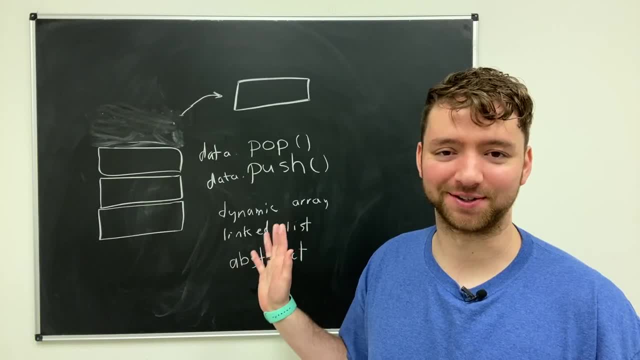 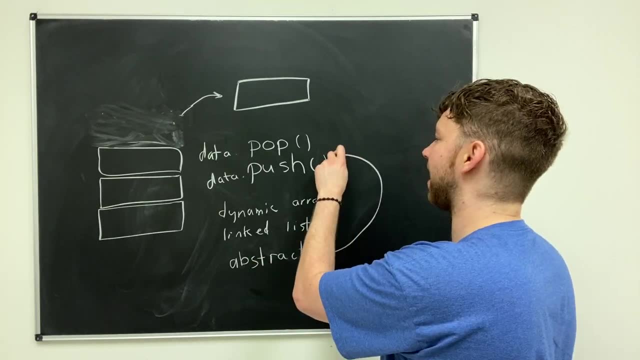 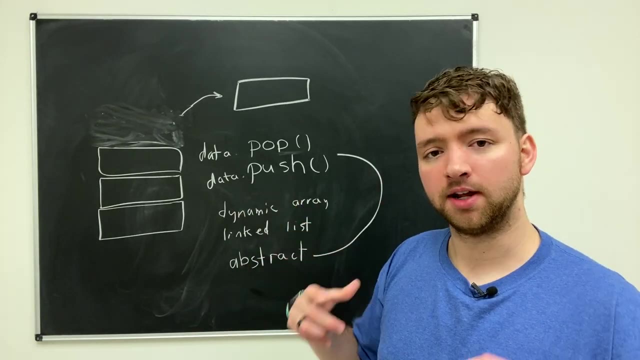 it into existence- And I'm not an artist, okay. But similar thing here, where we define behaviors a little bit more abstractly by just saying, hey, it has to have a pop method and it has to have a push method. The actual implementation can vary. So, for example, if you're doing a stack, you're 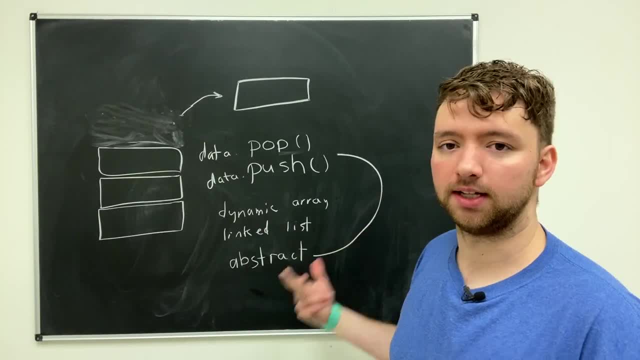 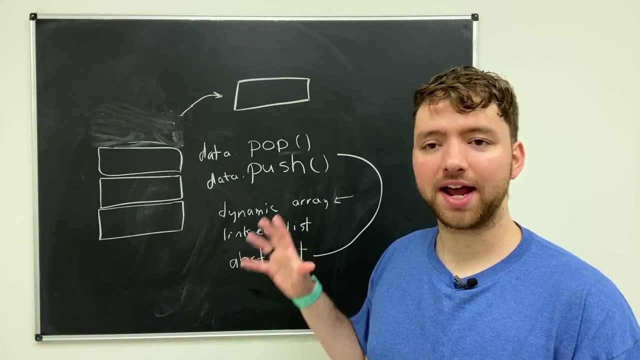 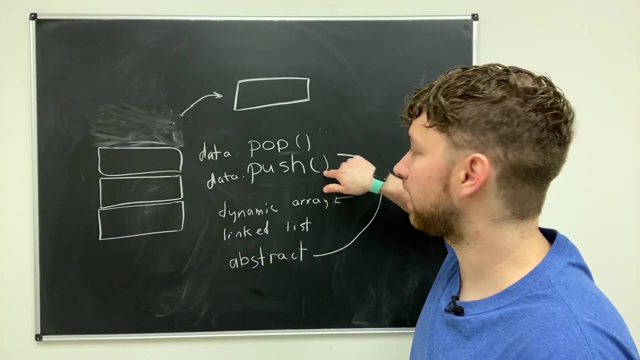 It could be a dynamic array, It could be a linked list. It's up to you guys to decide how you want to actually create a stack data structure. So the stack is less about a physical thing and more about a set of behaviors: The ability to push something on the stack and the ability to pop. 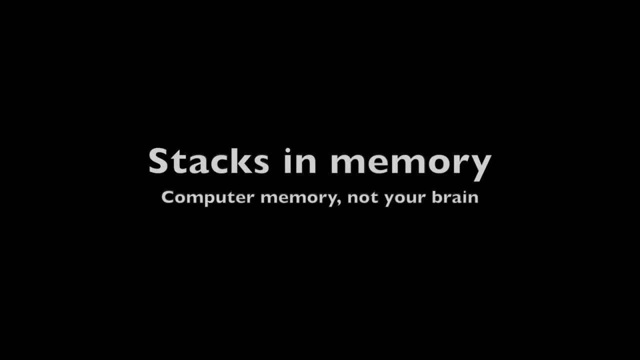 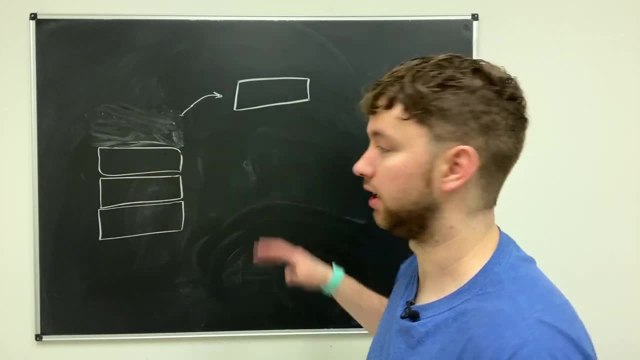 something off of the stack- Crazy. So let's start from the beginning and build this stack right here. I'm going to use this stack as a starting point And I'm going to use this stack to erase it and we're going to go from scratch. So the very first thing is we put our very first. 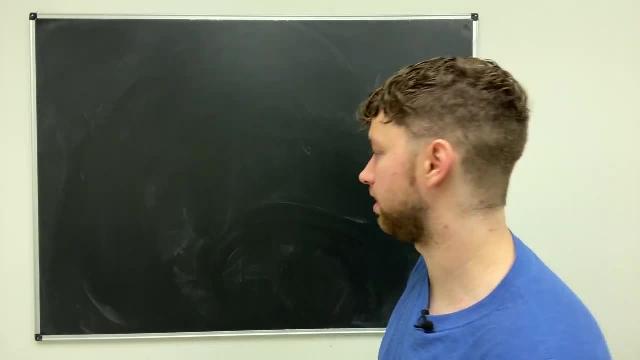 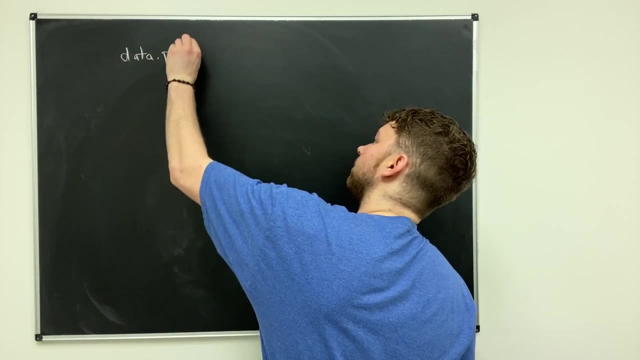 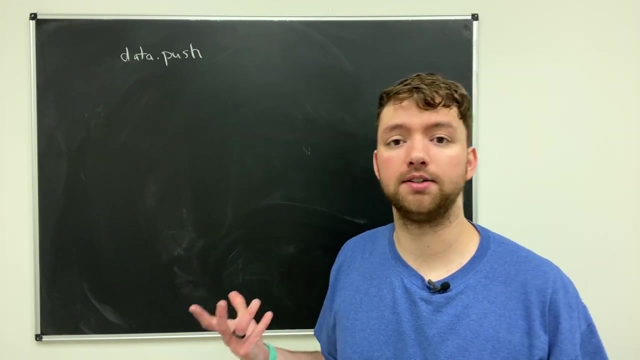 element, And to do this we invoke the push method. So here is going to be the actual method calls. So we'll say datapush, And instead of using the concept of books, let's just go with some other type of data, like integers. Let's say we push the number five. Well, we're going to see how you could. 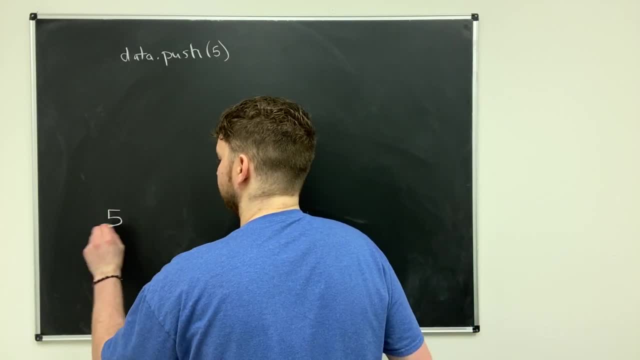 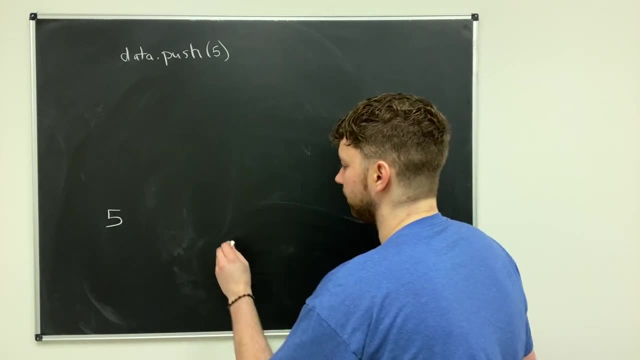 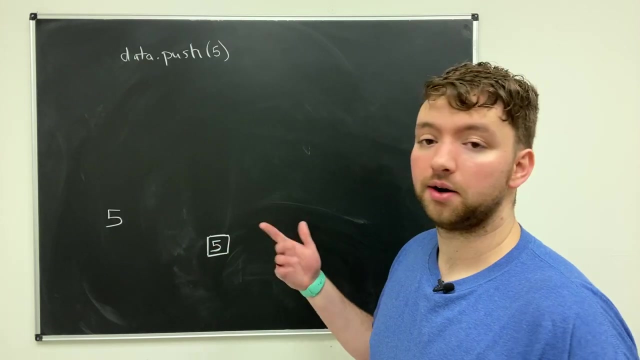 visualize this over here. So we're going to have the value five at the bottom of a stack, Then inside of our array it's going to look like so: One element, five. Now let's say we want to put another piece of 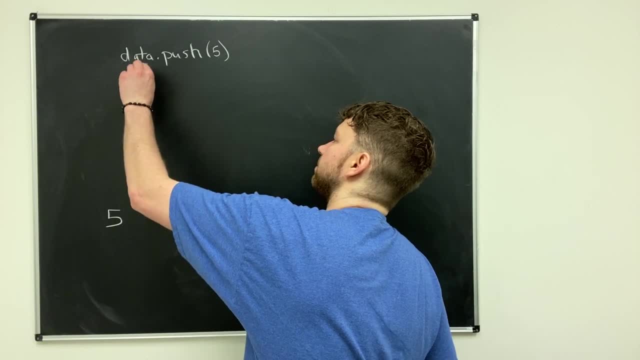 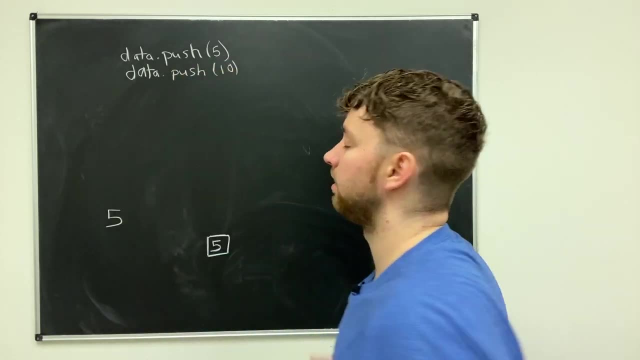 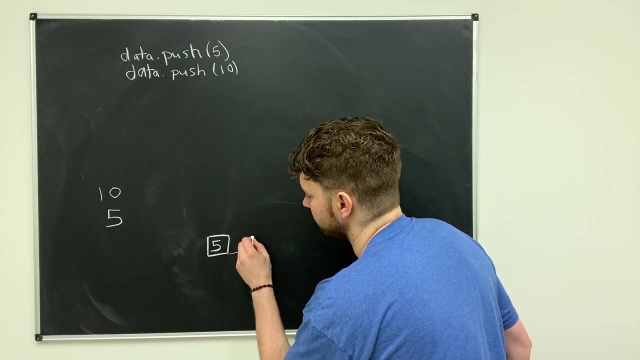 data on top of the stack. The way we would do that is we would say datapush, And this time let's pass in 10.. So, 10.. So this actually is going to be on top of this five and is going to be represented in the array. 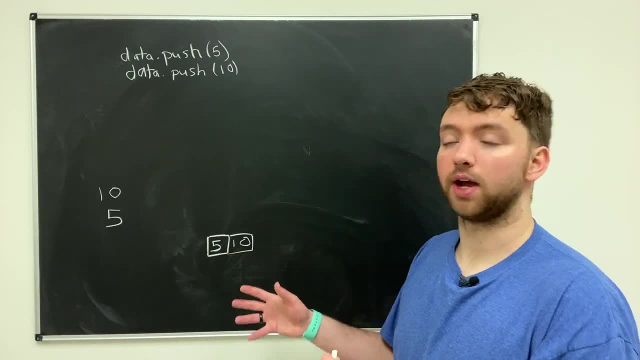 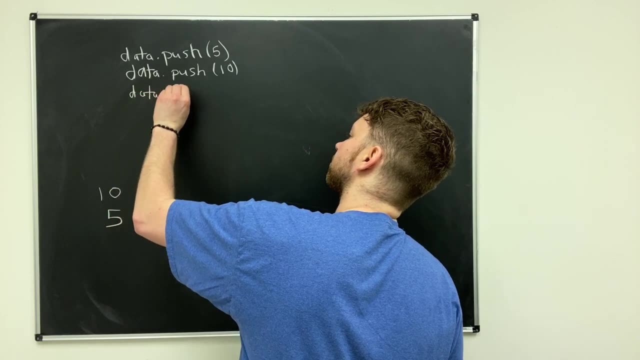 just with another element. So the length of the array is now two. Now let's add one more element in here, So we'll say datapush And let's pass in negative seven, just to switch it up. All right, 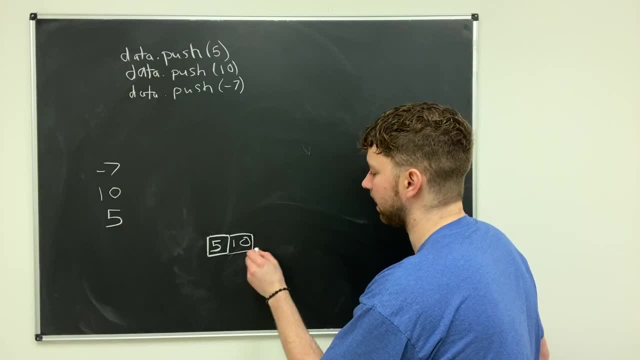 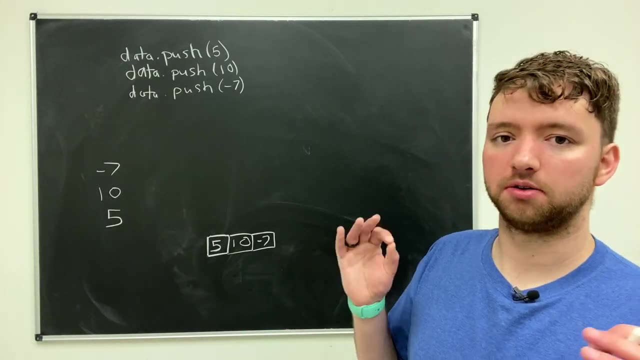 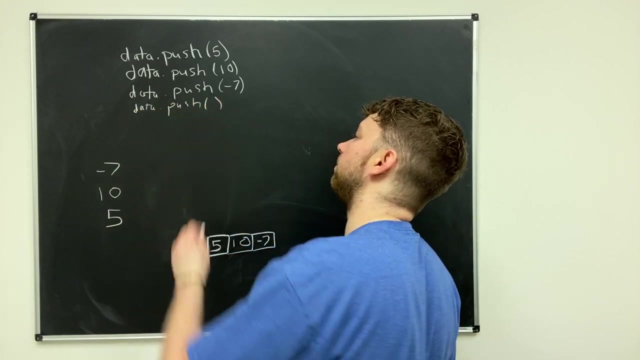 So this is going to go up here and we're going to have another element in our array, like so, All right, Let's do one more element and then we'll talk about pop. So let's say datapush And what number you guys want to put. You want to do positive seven, All right? Yeah, I like that. 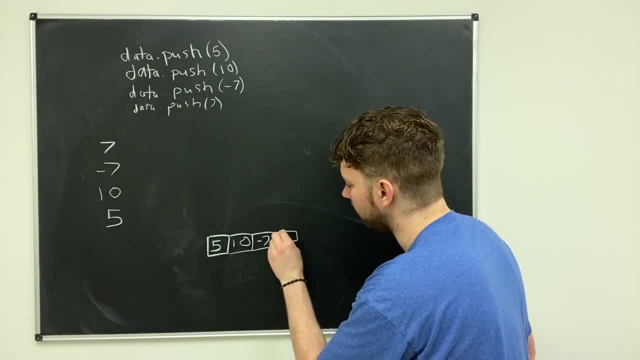 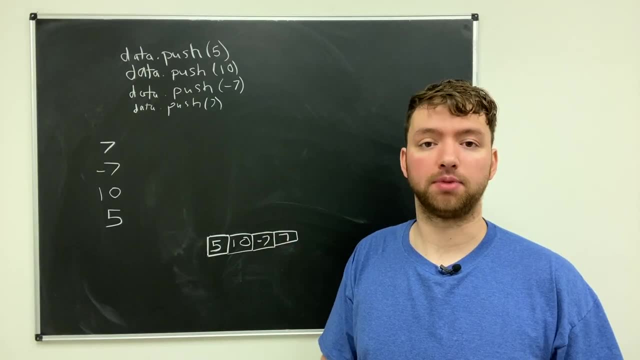 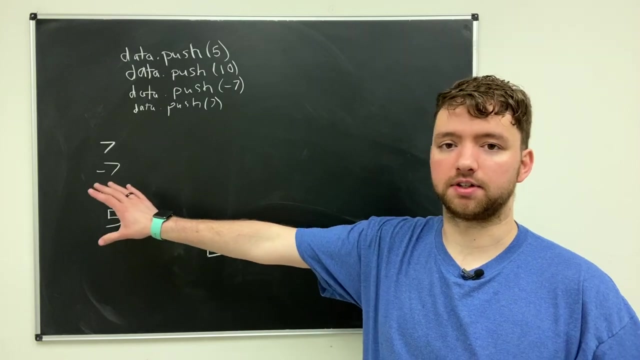 All right, So that's going to go there and that's going to go right there in our array. So now let's talk about the pop operation. So the pop operation modifies the stack. It changes the data of the stack. What it does is it will remove this element here. 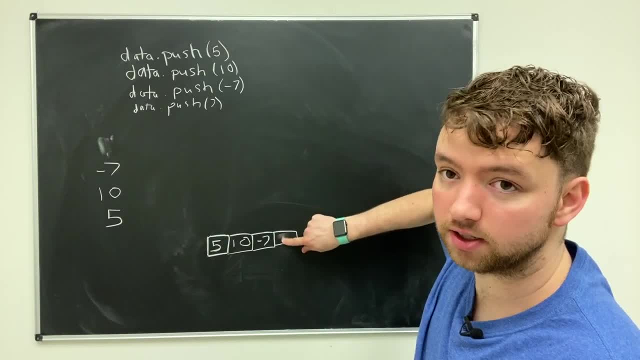 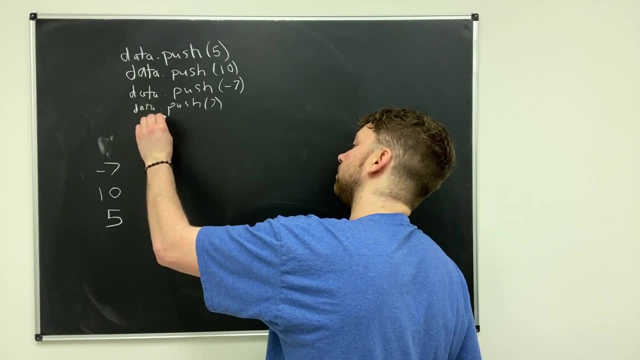 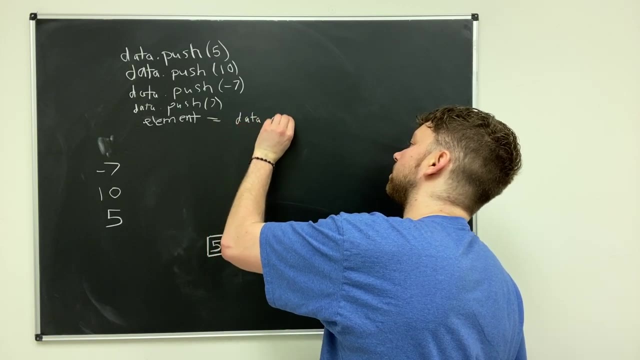 It'll remove it here and return it. So what that means is we can assign it to a variable. So the call to this would look like: so We would create some variable and then we would invoke datapop. We don't pass anything in, It's always going to grab that top element. 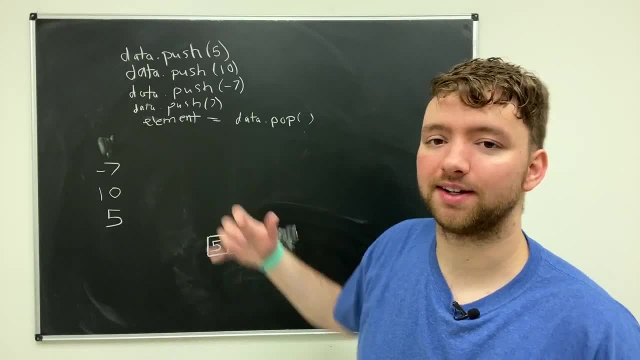 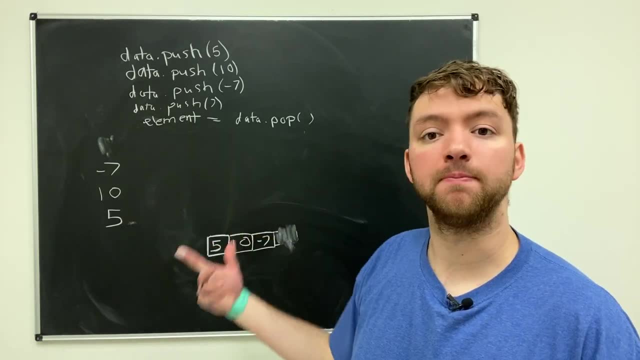 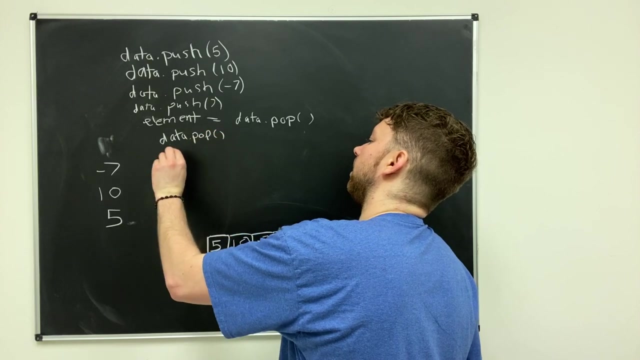 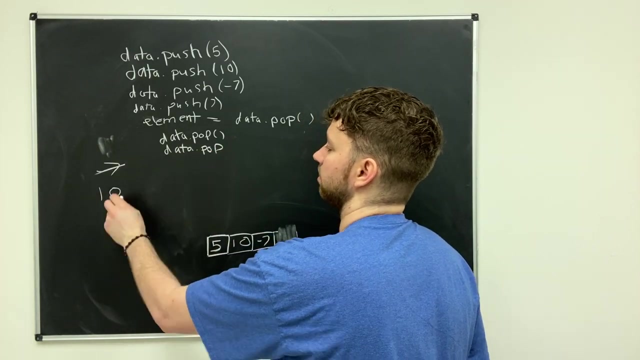 And now this variable element contains the value seven. So that is how a stack works. So if we wanted to get this element here, here's what we're going to do: We're just going to say datapop, Again datapop. So the first one will get rid of that number, The next one will. 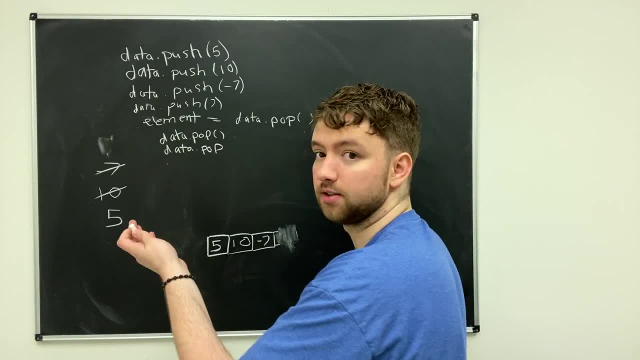 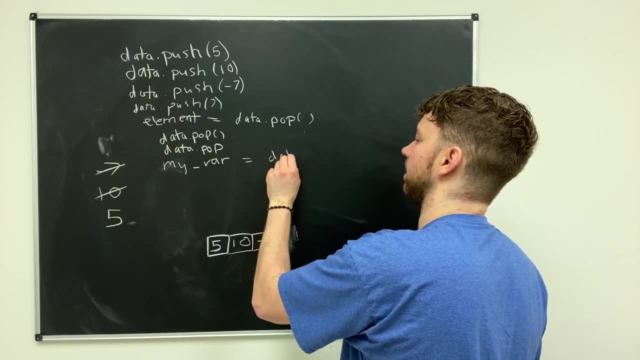 get rid of that number And then we do it one more time and we can assign this one to a variable- Let me think of some creative variable name- And this is going to be assigned datapop Now, if you don't actually need to use that data later, for example, in this case, the negative. 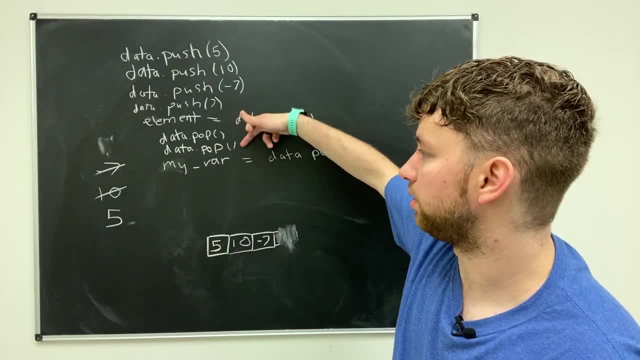 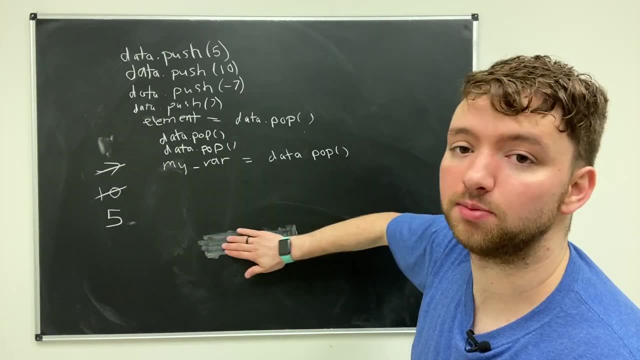 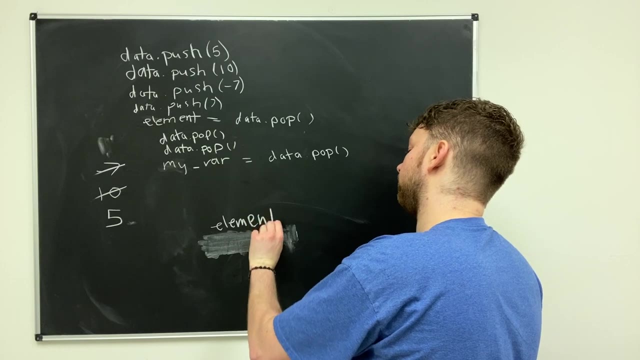 seven and the 10,. you can just invoke pop without actually storing that anywhere. But if you need to use it later, then you can assign it to a variable. Now our array is going to be empty, but we're going to have two variables available to us: Element, which is going to contain 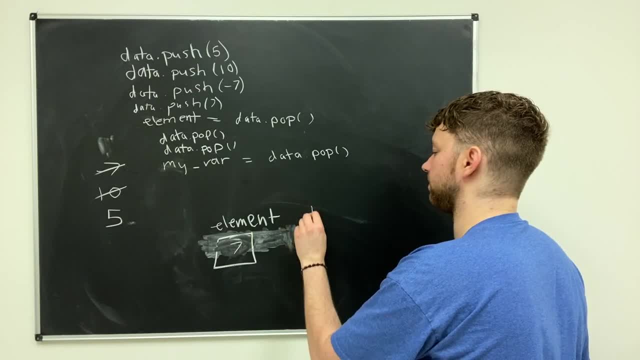 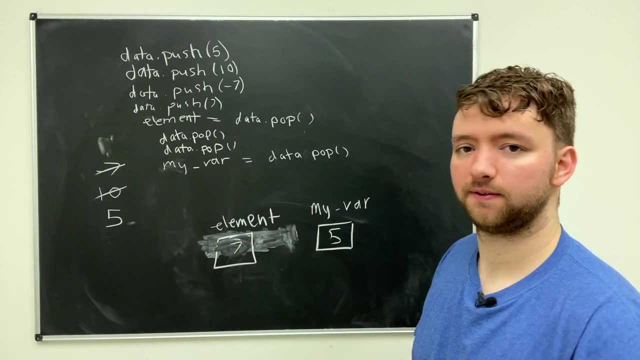 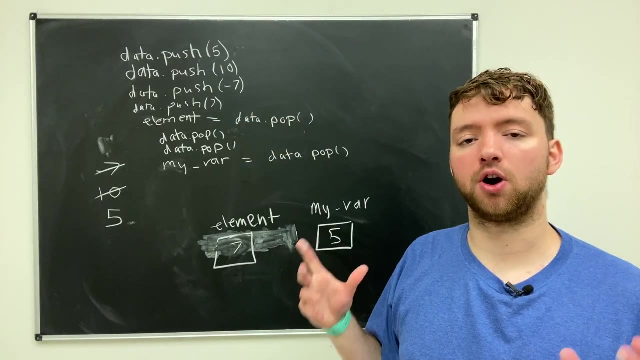 what was it? Seven? And then we're going to have this other variable, myVar, which is going to contain the value five. So cool, That sounded so unenthusiastic. So the push method and the pop method are methods that describe the operations, But if you are working inside of a programming, 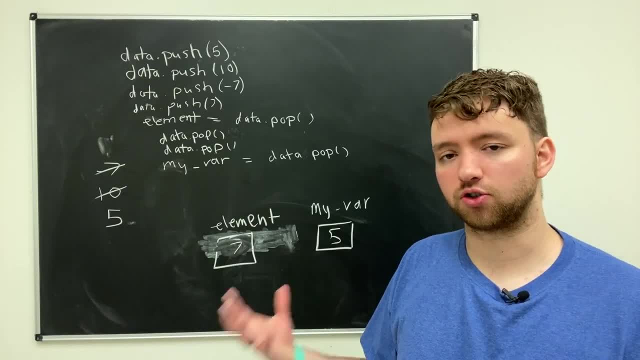 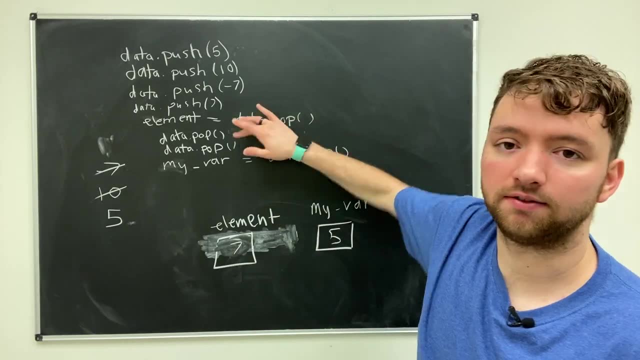 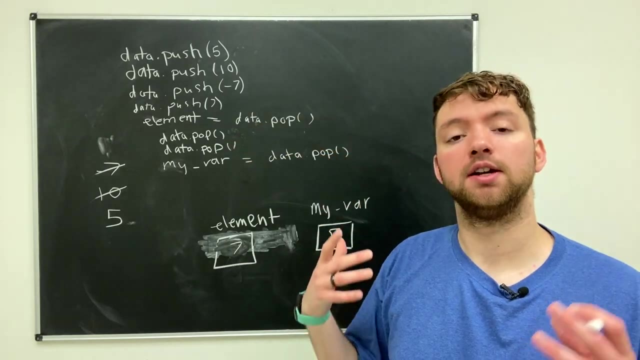 language. it's going to depend on whatever structure you are using. So if you were to use a list inside of Python, these methods are going to be different. If you are in an array list inside of Java or C sharp, these again are going to be different. So the actual method names: 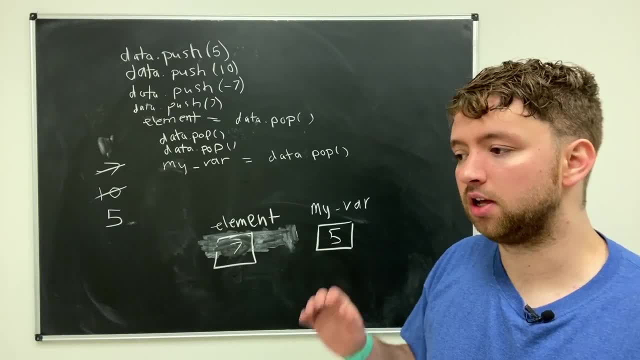 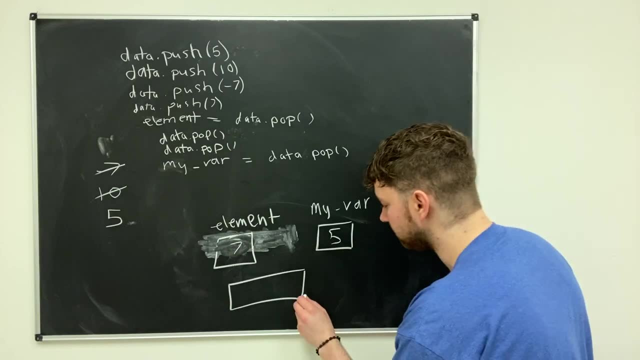 change, but the functionality stays the same. The way to describe this without using these names is basically the ability to add an element to the end of the collection and the ability to remove it and return it. So if you are working inside of a programming language, 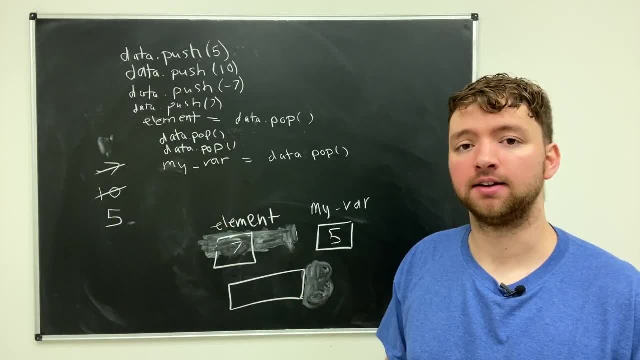 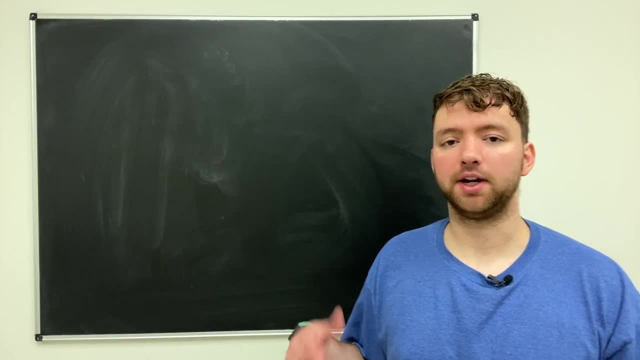 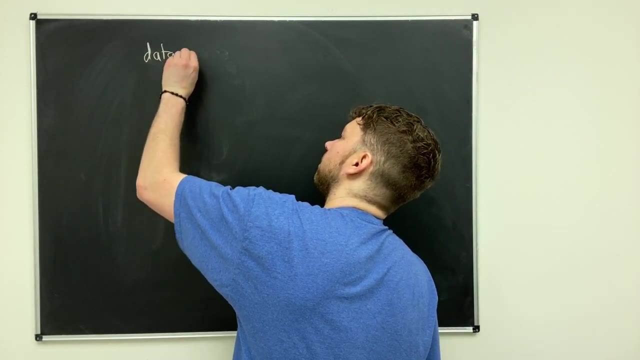 you can add an element to the end of the collection and return it. So those are the two general behaviors of a stack. Now let's talk about an example with Python. To create a stack inside of Python, we first create a list variable, So that's going to look like. so We would say, data. 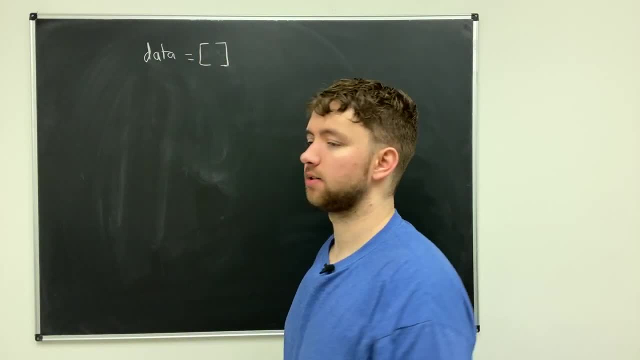 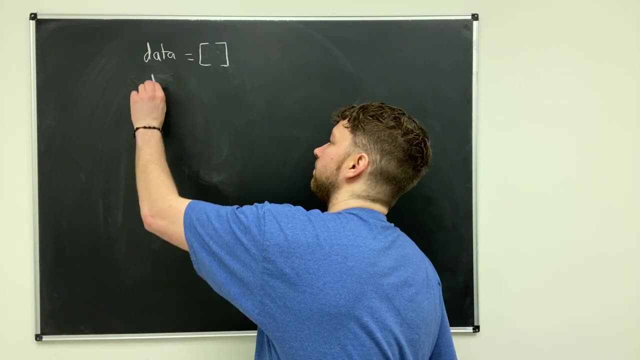 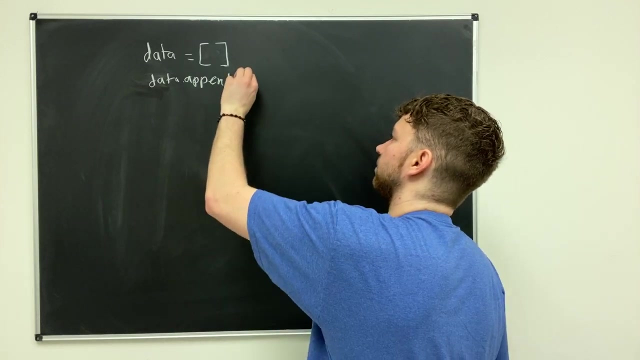 and we'll just assign it an empty list. Next up is the push capability, And with a list inside of Python, this method is known as append. So we would say data dot append and we would pass in some data, such as five. Now for the pop operation, Python, actually. 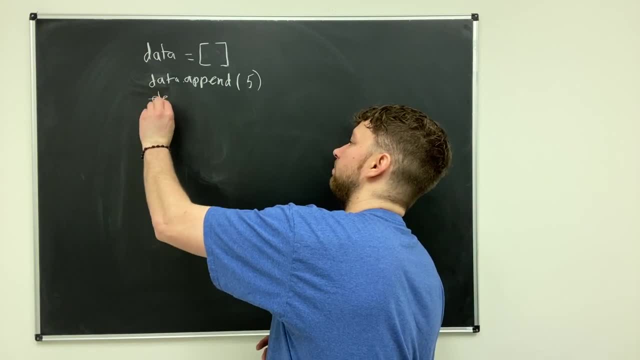 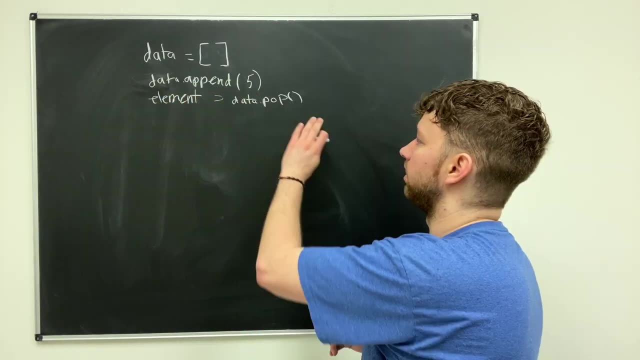 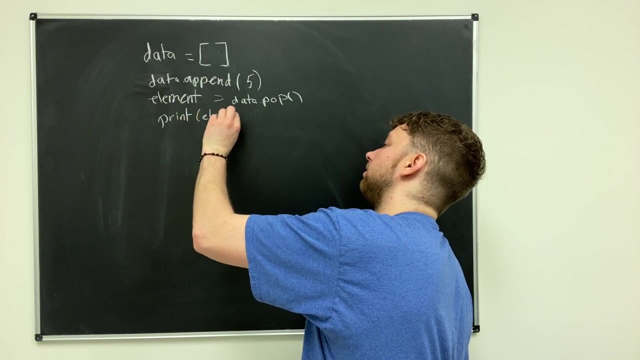 kept that name. So we could say something like elements or literally any variable name is data, dot, pop And that is a method call, And then what we can do is, if you wanted, you could say print and pass in element. So that is how you would do this inside of Python, but I'm sure 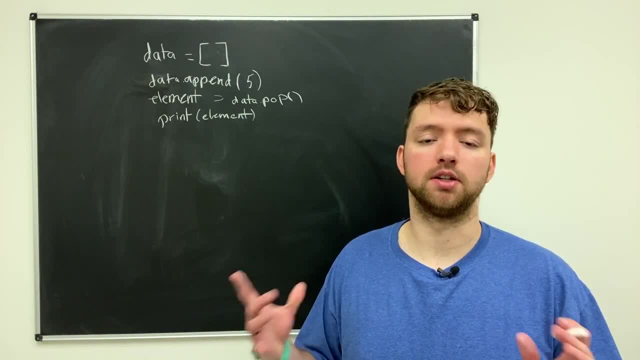 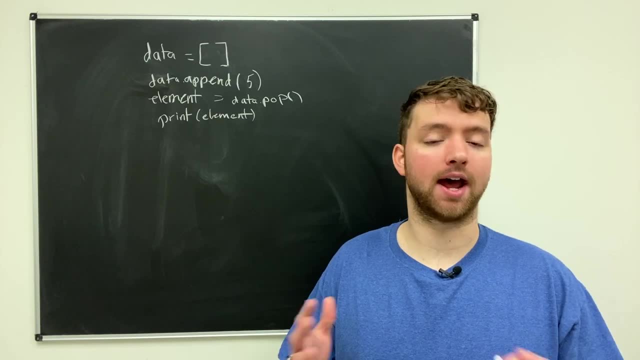 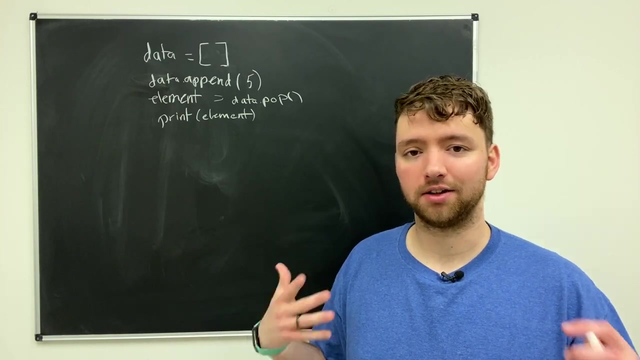 you're figuring this out in any of the major programming languages is going to be fairly simple. Now again, because a stack is an abstract data type. all it really cares about is that there's a push operation, and a pop operation Doesn't necessarily mean there can't be other things, So 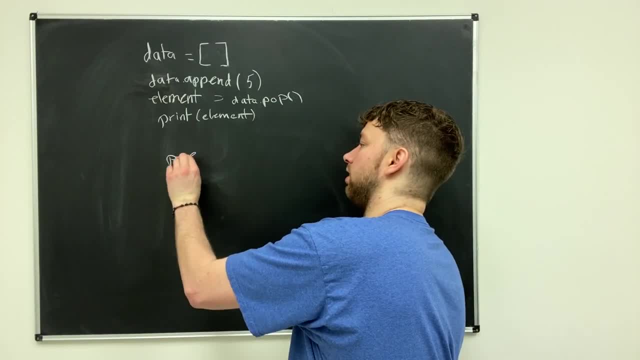 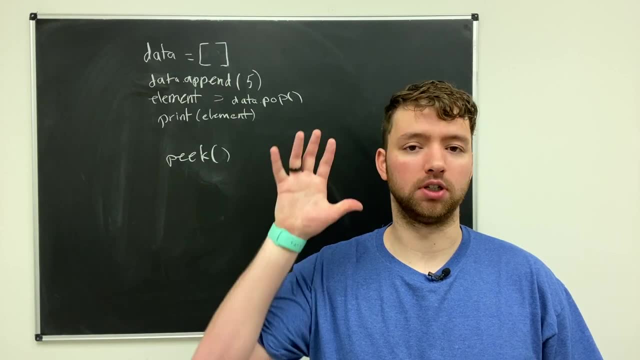 oftentimes there will be some variation of a peak method And what this will do is it will actually look at that top element without actually looking at that top element, So it won't actually look, actually popping it off of the stack. because if you have a stack, 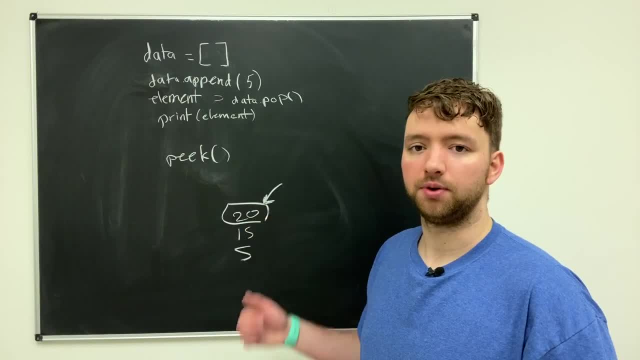 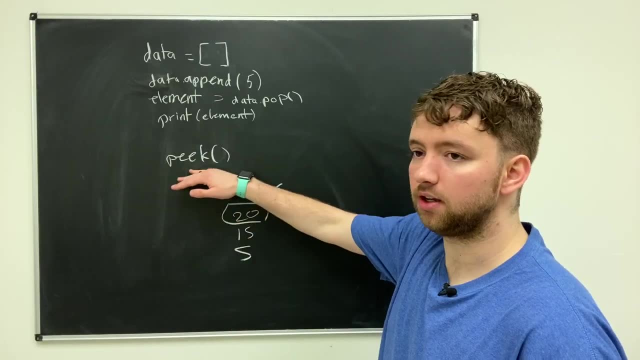 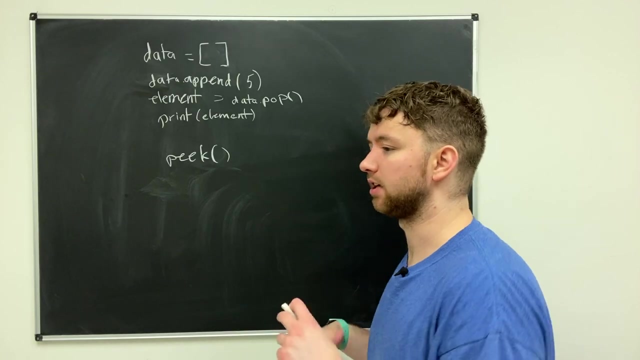 you might want to check to see what this number is right here without actually removing it. so that's sometimes called peak. if we're just talking about the abstract data type, you would say peak. but different languages are going to have different names, so a very universal way to do a peak would basically be to grab the 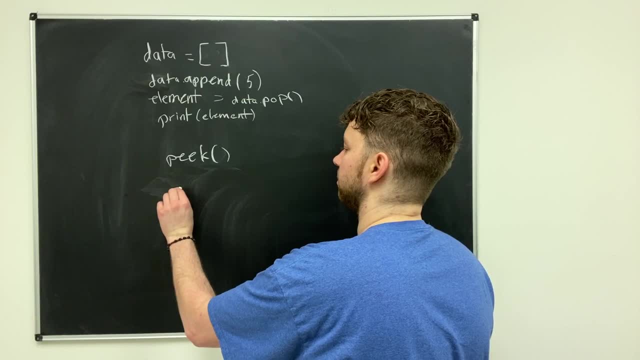 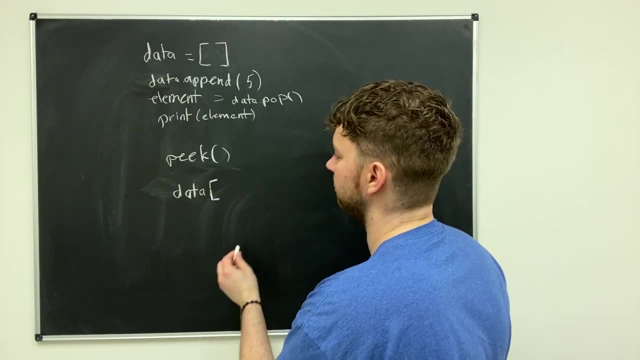 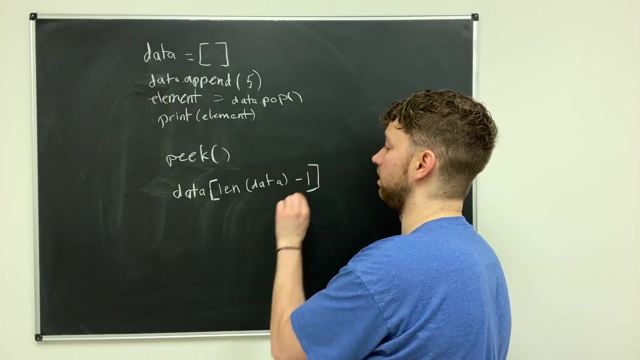 element at the last index. so in this case what we would do is we would say data, and then we would use array notation or just square brackets, and inside of here we're going to say the length of data minus one, and that's how you would get that last element. 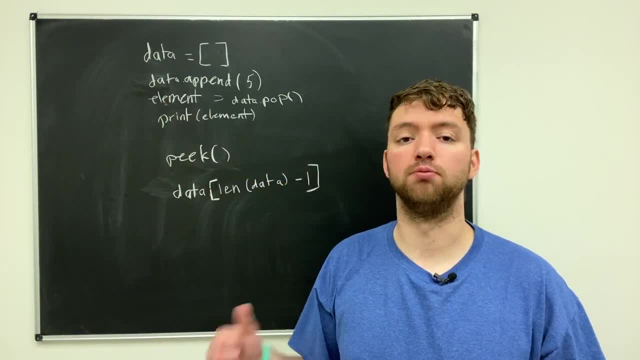 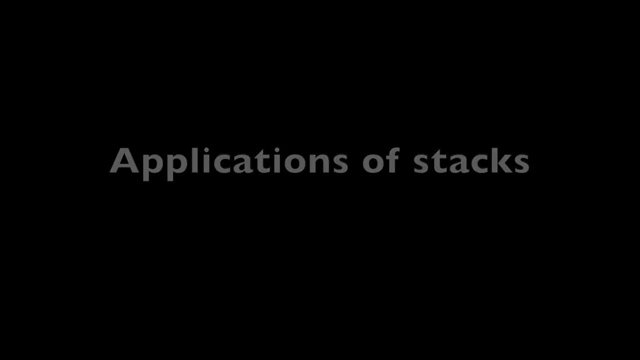 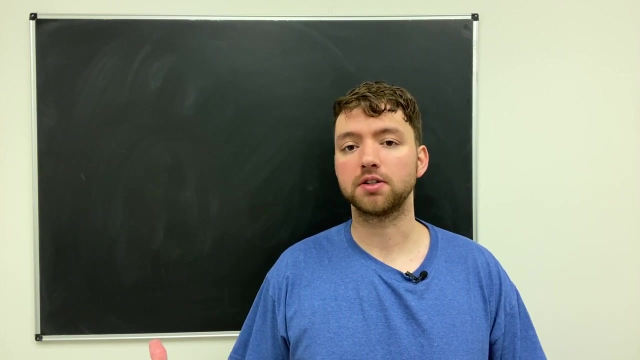 you could assign that to a variable, just like we did here, but it's not actually going to remove it from that list, so the list stays unchanged. so we talked about stacks and we understand them conceptually. when would you actually want to do something like this? well, there's various 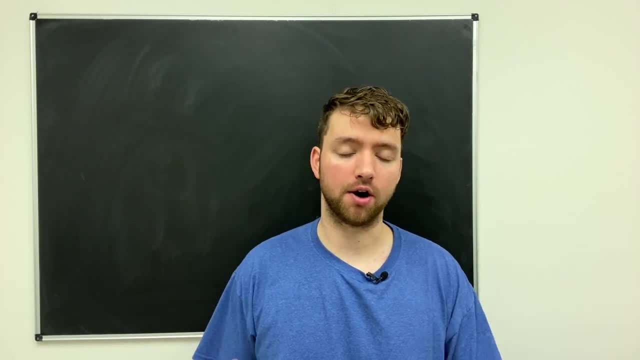 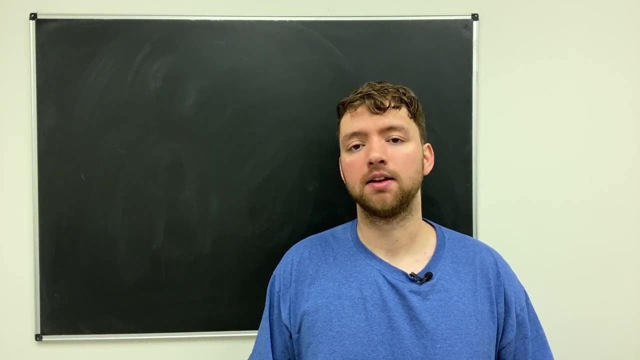 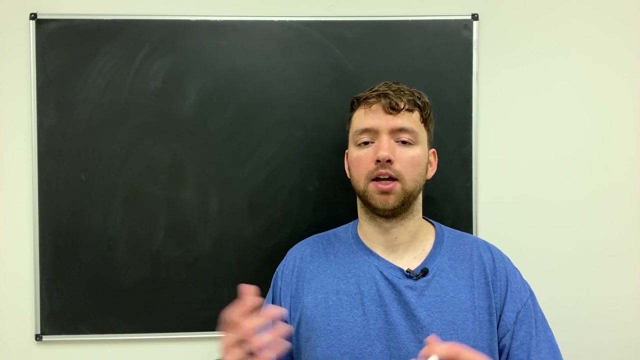 ways that this is used already. so, for example, a call stack. basically anytime you invoke a function in your code, that gets added to a stack. so when that function finishes and returns, we basically pop that function off of the stack and return to where we were. so there's a portion of memory known as a stack. 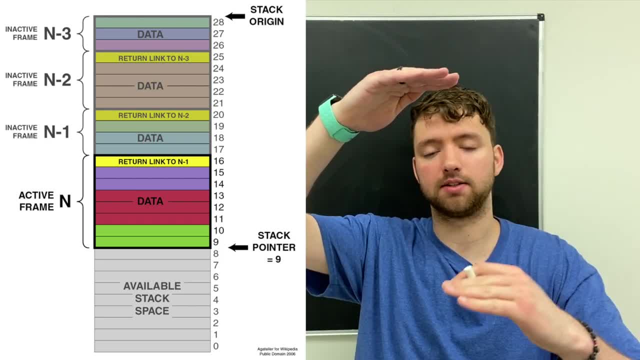 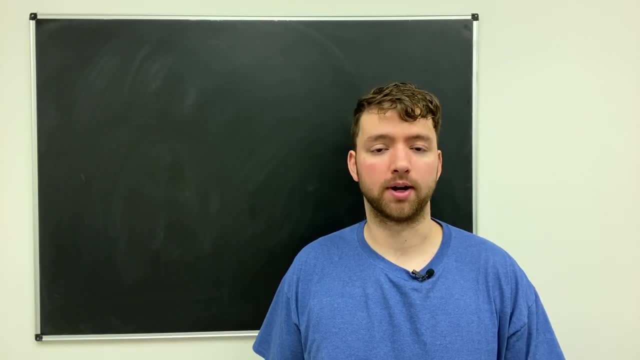 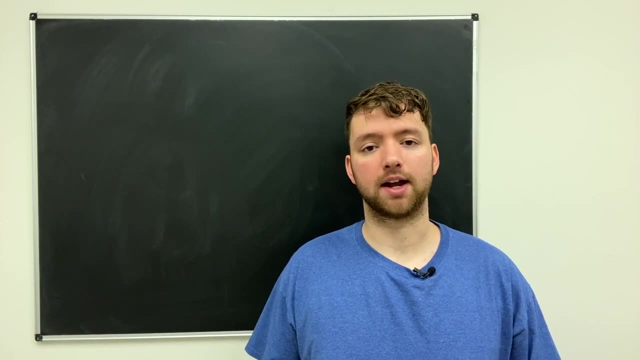 and this is actually like an upside down stack, so we add elements this way, grows this way, and this is just a portion of memory that is used for various things. so if you want to know more about that, just look up stack memory or something like that, and you'll be able to find information on that. another common use of the stack: 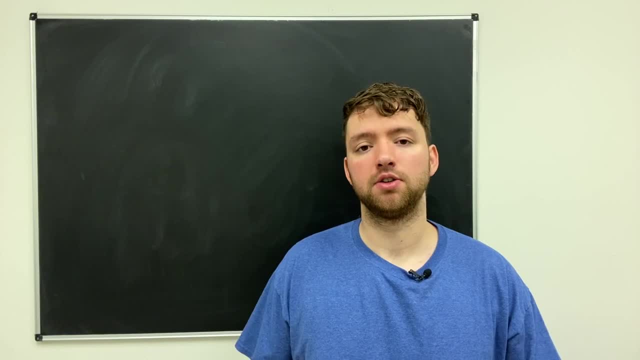 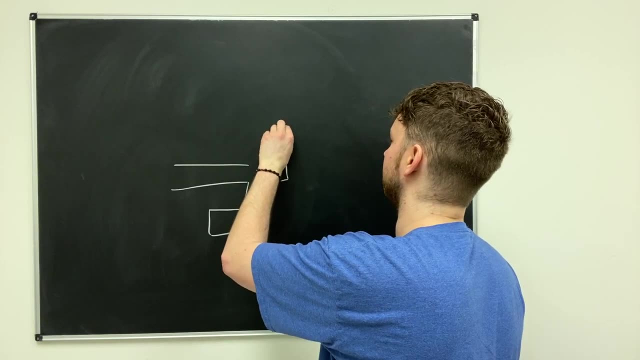 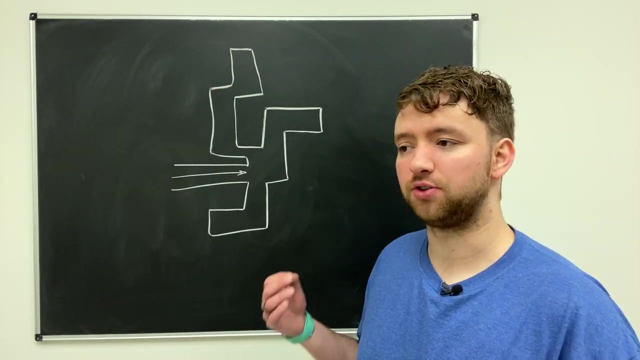 data structure is to do something known as backtracking. so if you imagine you had like a maze, i'm gonna try not to draw a swastika here and here you are. well, if you want an algorithmic way to describe how you would solve this, you basically go down a path. let's just 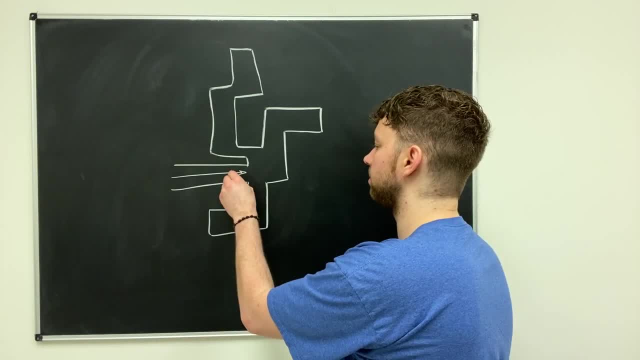 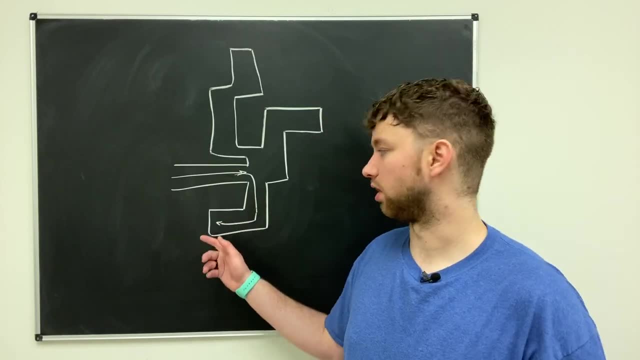 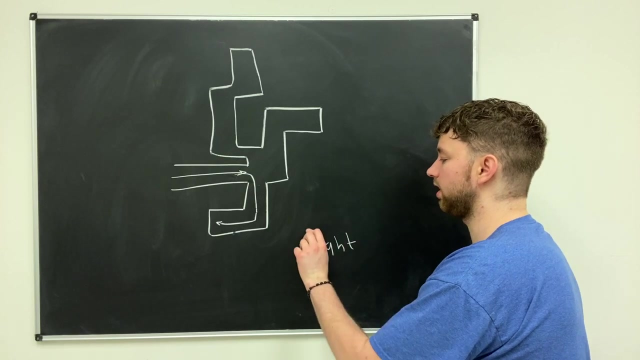 say, you always go to the rightmost path first, so you go right and then you go. what would that be? that'd be right again, and oh, you hit a wall. that doesn't work. so if you put those right operations in a stack and you basically had a list like: so right. 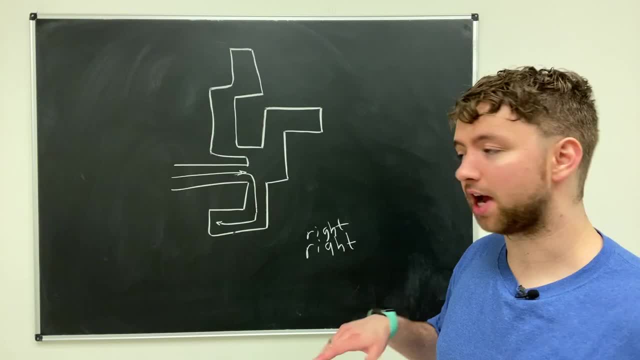 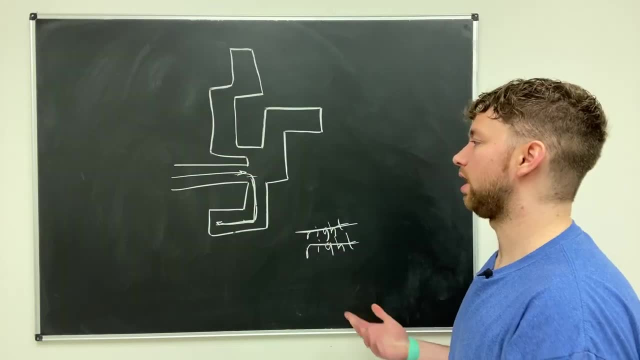 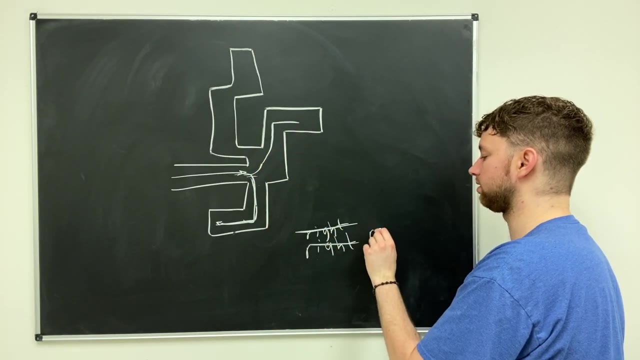 right and then you hit a wall. then you just back track, You pop those off the stack and say, hey, we need to back up, and then we need to back up again and go this way. Now it looks like we might go left and keep going left until we go right. So now the stacks going to look like this: Left. 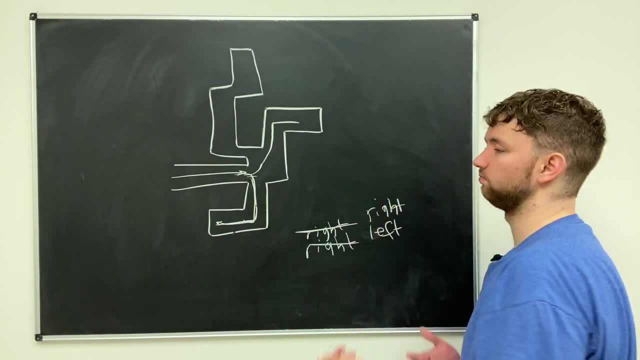 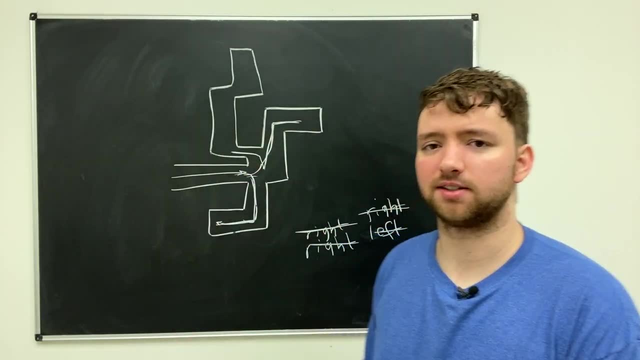 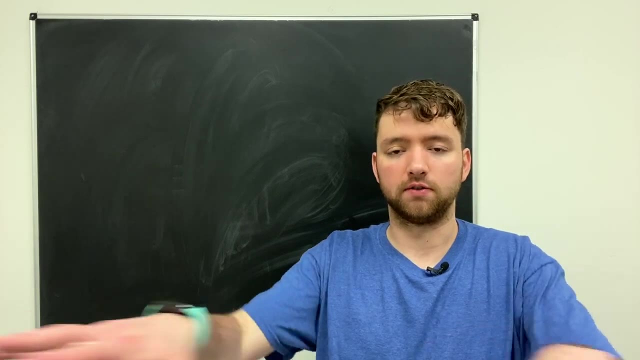 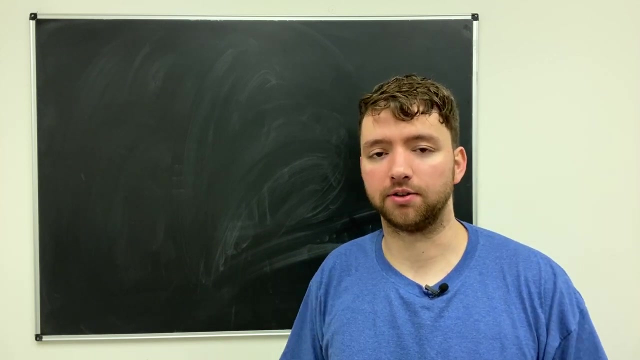 and then right, Mmm, that's not working out either, so you pop those off the stack and backtrack to where you were. Anyways, this is getting like really ugly. but basically the backtracking is an approach to solve various paths in code. I actually did a video on solving mazes in Java inside of my 30 days of Java. 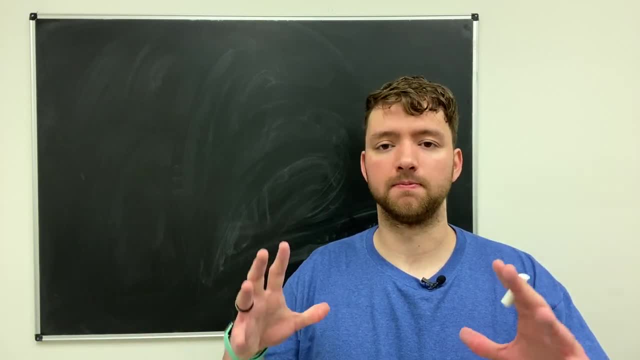 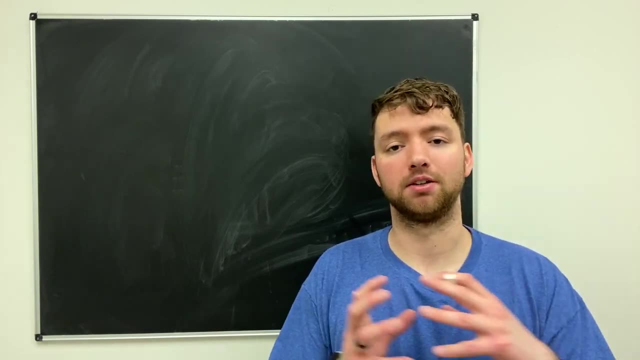 series, if you're interested. We build out a maze structure using ASCII characters and we basically tell the computer to start at a position and end at a position and it will basically follow these different paths. It's something you can build recursively or iteratively and we're going to get 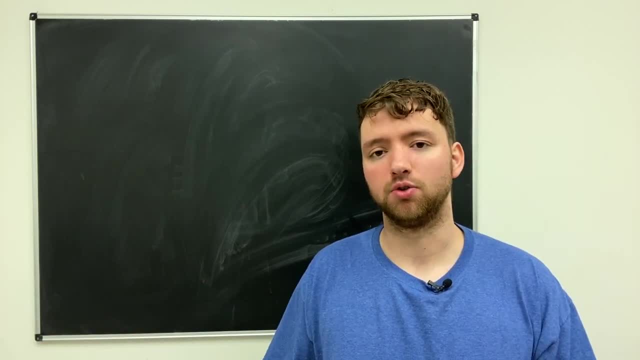 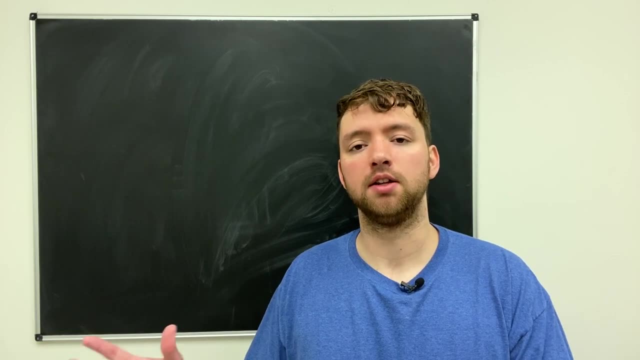 into this in a minute. The difference is there in the future. but basically it's a really cool way to make the computer try all possibilities and if it knows a direction doesn't work then it's going to back it up and try a different path. So that's your.